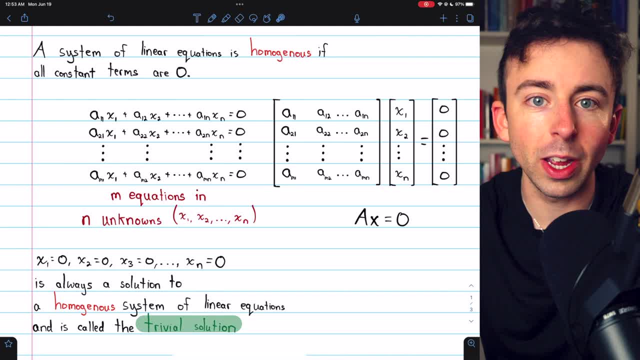 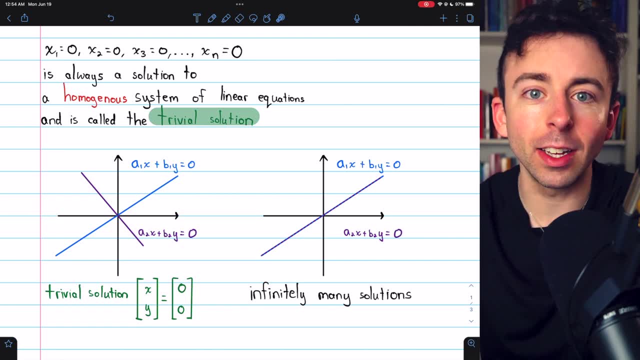 the zero vector. So it is a solution to the equation. It's the trivial solution. The case where our homogeneous linear system has two unknowns is easy to sketch because those are lines. right, We've got an X and a Y, two unknowns, so we're talking about lines. This is what the 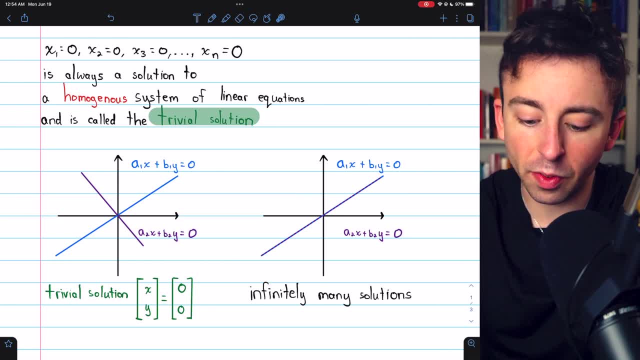 trivial solution looks like. in that case We've got two unknowns: a1x plus b1y equals zero, and then this other equation, a2x plus b2y equals zero. The trivial solution is where these lines intersect at the origin. 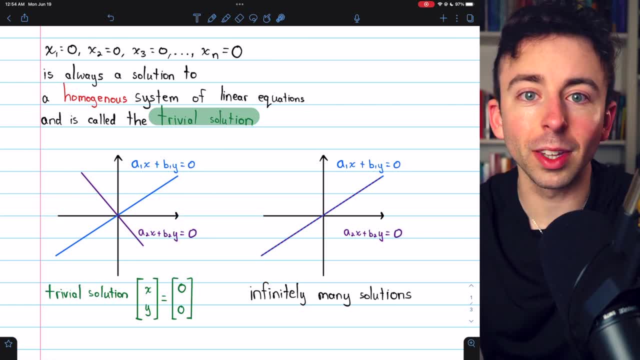 Because the constant terms are 0, the y-intercepts of both lines are 0. If we set x and y equal to 0, we get a solution. The only other possibility is that there are infinitely many solutions if the lines exactly coincide. 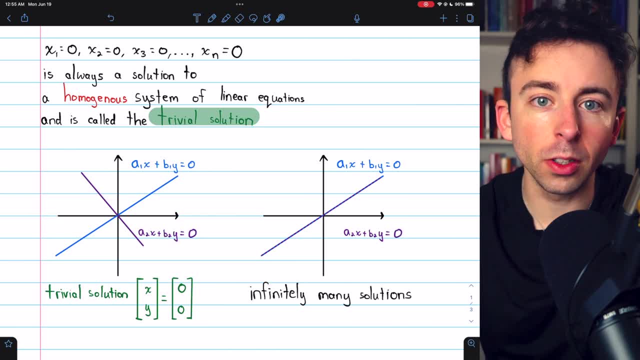 Of course, the only way to get there to be no solution would be if the constant term was not 0. That way we could shift one of these lines up, But then we wouldn't be talking about a homogeneous linear system, because the constants got to be 0.. 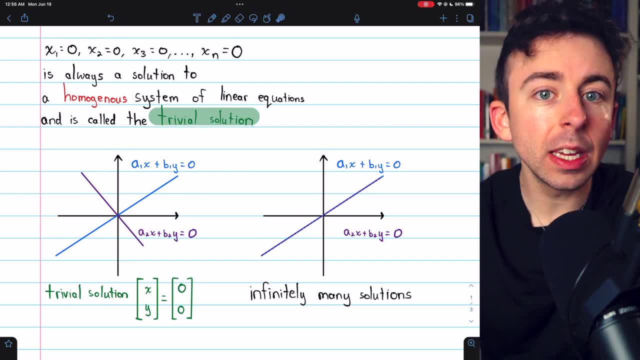 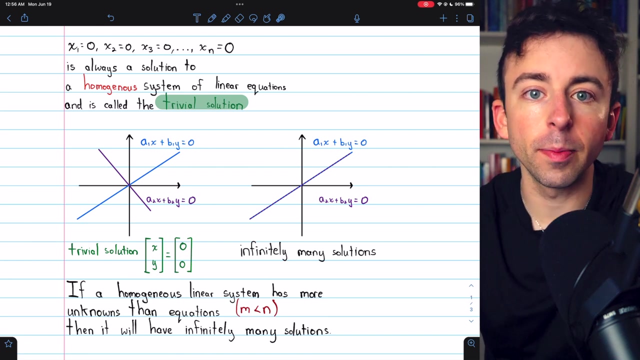 And this is the case for any homogeneous linear system. even if it has more than two unknowns, They will always either have only the trivial solution or infinitely many solutions. For a homogeneous linear system of equations, these are the only two possibilities. There is one situation where it's very easy to see that a homogeneous linear system will have infinitely many solutions. 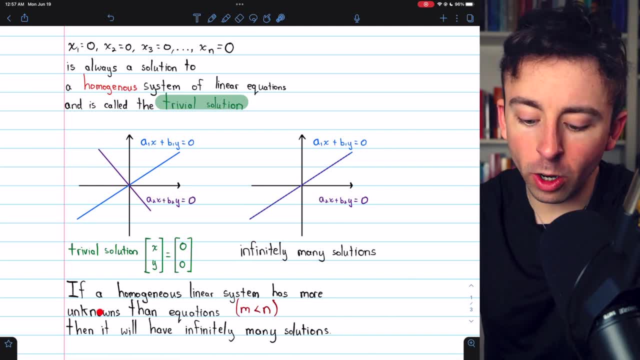 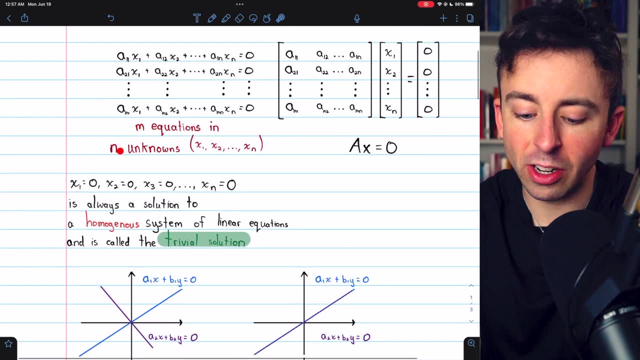 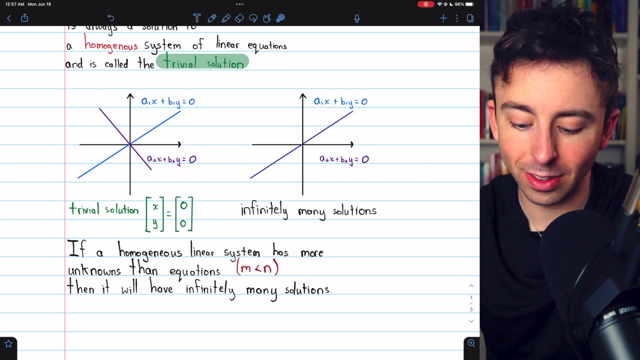 Which is if the system has more unknowns than equations. In terms of the letters we were using before, we had a linear system with m equations and n unknowns. So if m is less than n, if we have fewer equations than unknowns, then for sure our linear system is going to have infinitely many solutions. 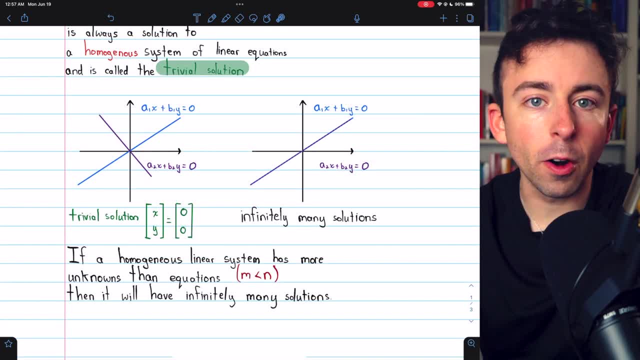 In these cases we have a solution. In these cases where there's more unknowns than there are equations like, for example, maybe there's two equations in four unknowns. two equations is not enough to determine the values of four unknowns. 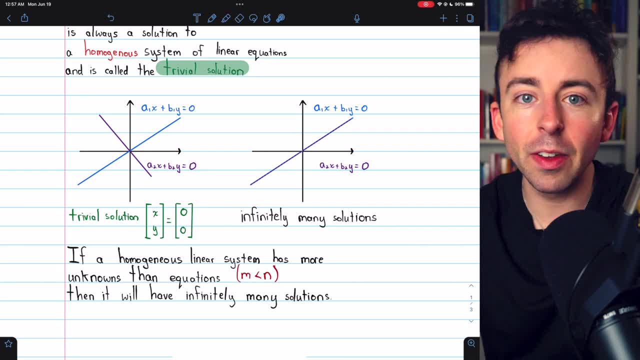 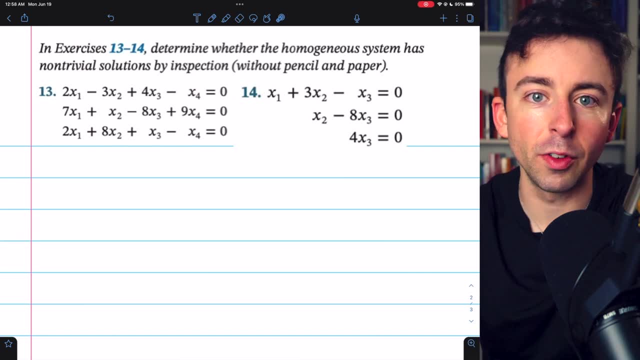 And so that would leave at least one free variable, giving us infinitely many solutions. Let's finish with a few examples from Howard Anton's Linear Algebra textbook- Link in the description. if you want to buy the book, it's great. In these first two exercises we want to determine whether the homogeneous system 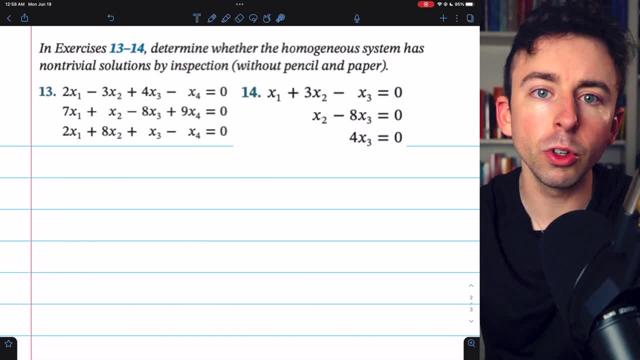 has non-trivial solutions by inspection, Which means we should just be able to look and figure out if it has non-trivial solutions or not. Let's look at 13.. Here we have three equations. We might say m equals 3.. 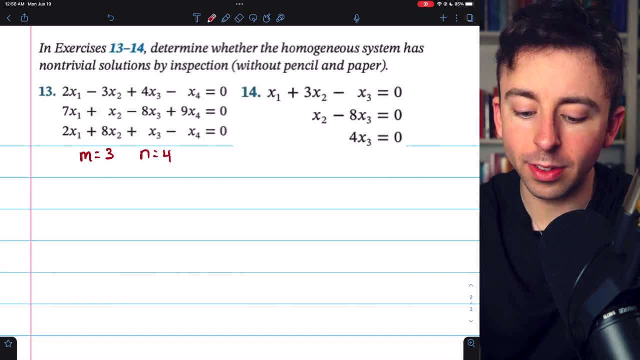 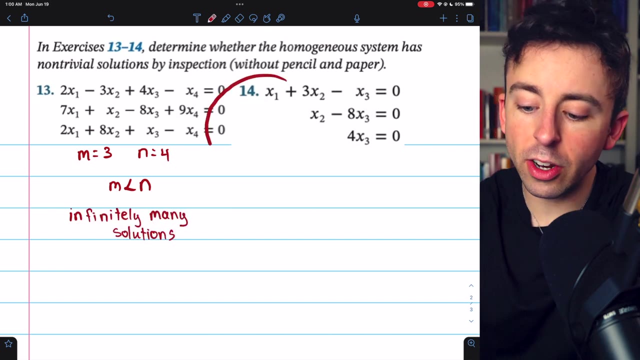 However, we have four unknowns: x1 through x4. So since we have more unknowns than we have equations, it's guaranteed that this homogeneous linear system will have infinitely many solutions. In equation 14,, on the other hand, we've got a homogeneous linear system, 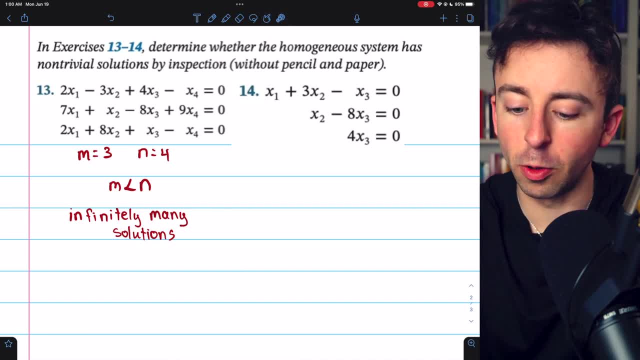 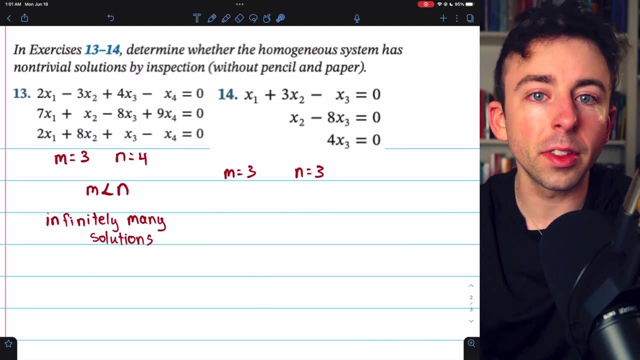 It's homogeneous because all of the constants are zeros And we see that it has three equations and it has three unknowns. So we can't immediately say that there are infinitely many solutions Just because the number of equations and variables are the same here. 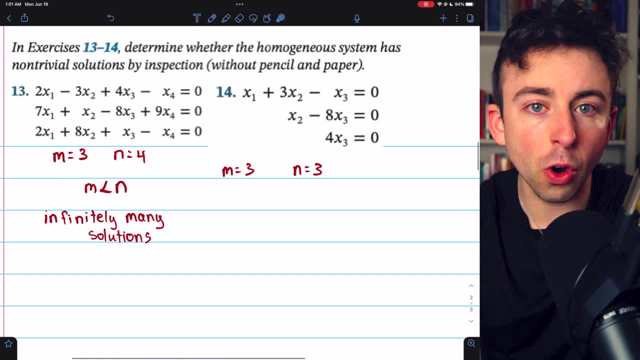 doesn't mean that this linear system for sure only has the trivial solution. However, it is pretty easy for us to check that indeed it does only have the trivial solution, Starting with this last equation: 4x3 equals 0.. That implies that x3 equals 0. 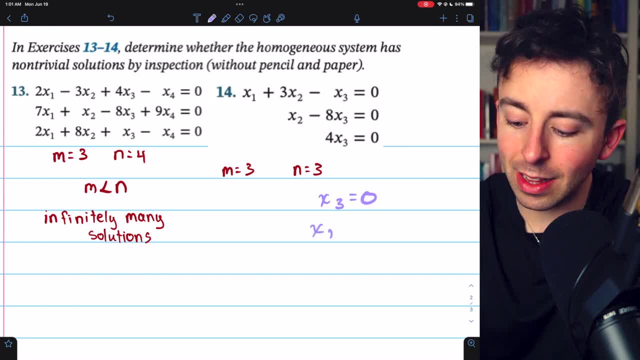 But then if we plug that into the second equation, that means that x2 minus 0 equals 0. Which of course means that x2 equals 0. But then if we plug x3 equals 0 and x2 equals 0 into the first equation, 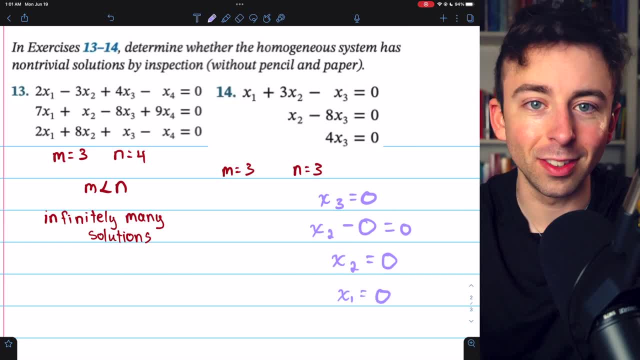 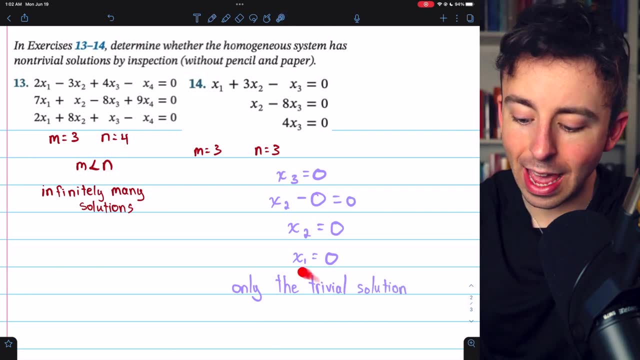 we get that x1 also equals 0. So while exercise 13 had infinitely many solutions, exercise 14, we only have the trivial solution to this homogeneous linear system, And I guess I did break the rules by writing some stuff down, but that's just for clarity. 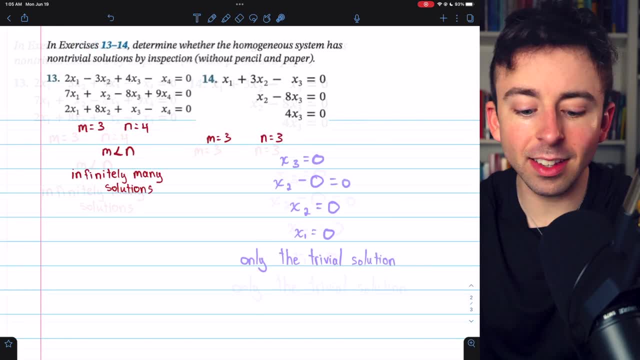 It's very easy to do these without writing any of this down, And since the system in exercise 13 has infinitely many solutions, if you were to perform Gauss-Jordan elimination on the augmented matrix for the system, you would end up finding that you have at least one free variable. 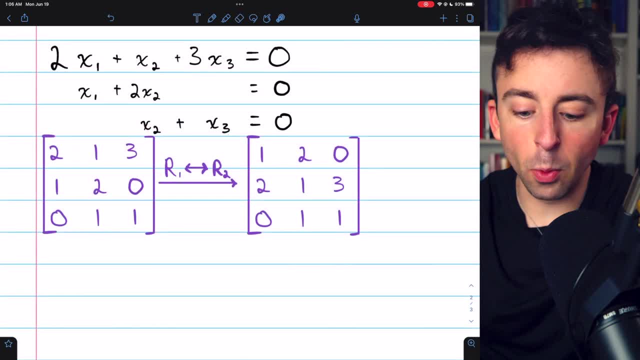 which indicates there are infinitely many solutions. Let's do one more example. Here is another homogeneous system of linear equations. Let's go through the process of solving it And we'll basically use Gaussian elimination to do this. Link in the description to my lessons on Gaussian elimination and Gauss-Jordan elimination. 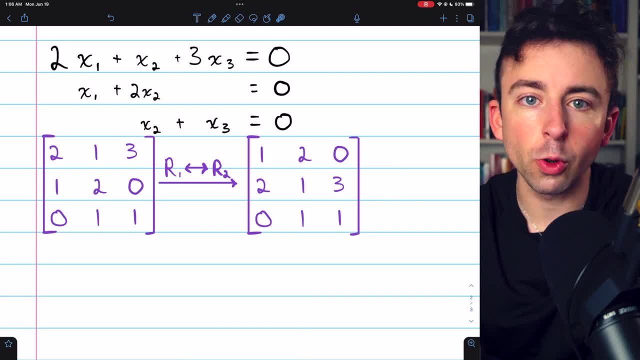 if you need a recap, This matrix here is the coefficient matrix for the system. Now, I've chosen not to include constants in the matrix because, no matter what operations we perform, the column containing the constants is still going to be all zeros. That's just a characteristic of homogeneous linear systems. 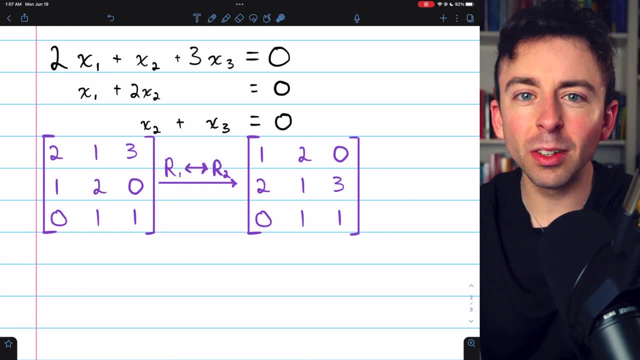 That last constant column will be all zeros, So it's not really necessary to include it. So we'll just work with the coefficients and be sure to remember that our constants are not here when we get to the end. My first step is going to be swapping rows 1 and rows 2.. 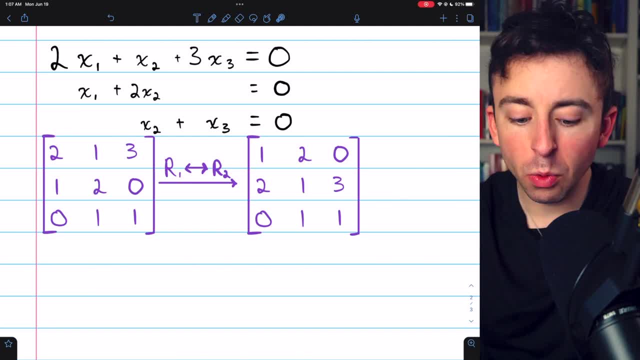 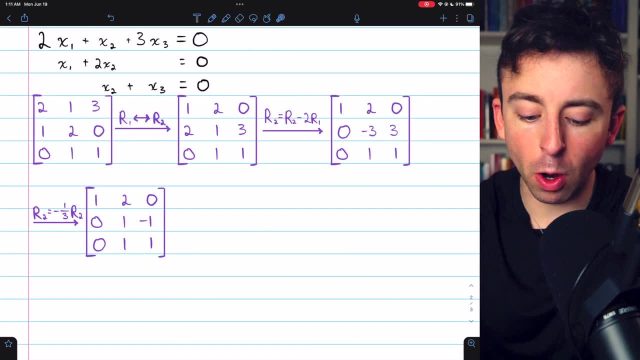 That way I get a leading entry of 1 at the top. We could have also multiplied row 1 by a half, but I'm trying to avoid fractions to keep our solution nice and clean. Swapping rows 1 and 2 gets us here. 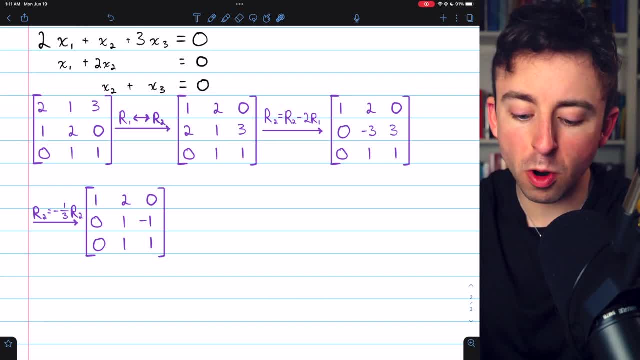 at which point we can subtract two copies of row 1 from row 2, in order to turn this entry below the leading 1 to a zero, We of course also have to subtract 4 from 1, which gives us that negative 3.. 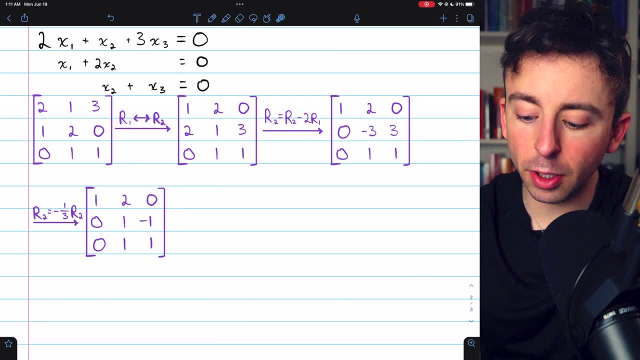 Now to turn this entry into a 1,, we can multiply row 2 by negative 1 third, which isn't actually going to introduce any fractions, because that, of course, plays nice with this other entry as well. Multiplying row 2 by negative 1- third gets us to this matrix here. 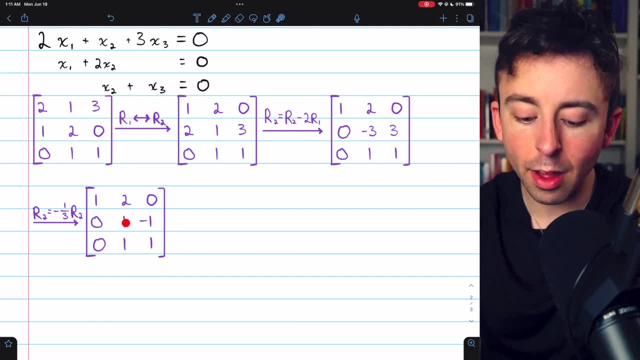 Now we can simply subtract row 2 from row 3, in order to turn this 1 into a zero. So we do row 3 minus row 2, that gets a zero there, and then 1 minus negative 1, is positive 2.. 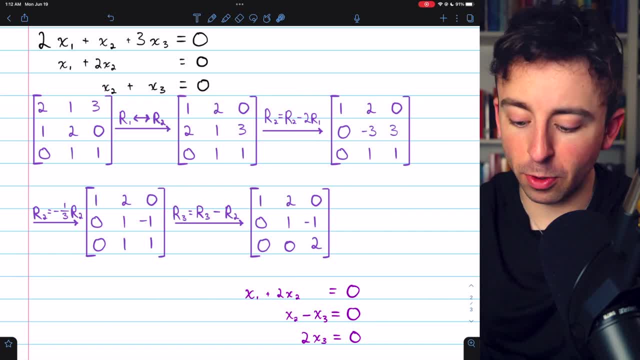 Now we can write the system of equations that's represented by this coefficient matrix. It's not quite in row echelon form technically, because we have a 2 here instead of a 1, but it's pretty darn close and the system is easy to solve now. 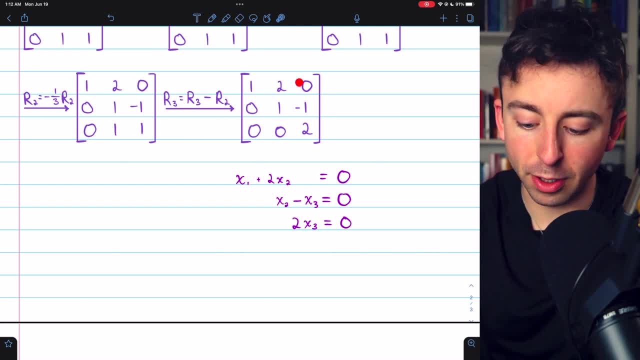 This is the homogeneous linear system that we've got now. Remember, this matrix represents coefficients, The constants are all zero And it's fairly quick to see that the trivial solution is the only solution to this problem. So in this linear system, 2x3 equals 0 means that x3 equals 0.. 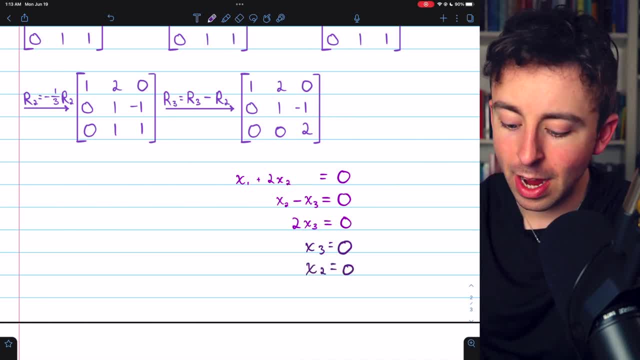 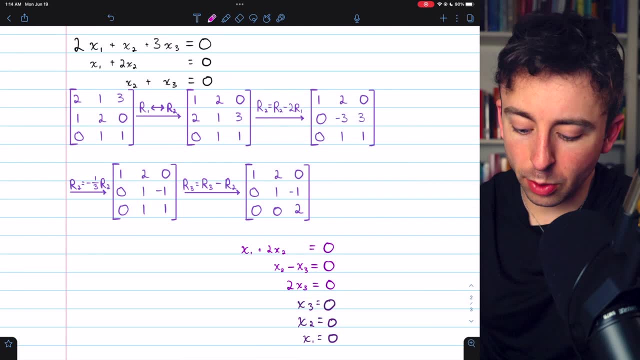 Plugging that into this equation gives x2 equals 0. And then plugging x2 equals 0 into the first equation gives x1 equals 0. So in this case we only had the trivial solution. I'll also point out that the number of equations 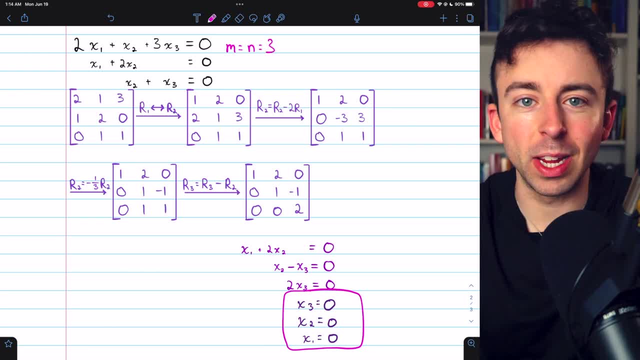 and the number of unknowns in this system were both 3. So we wouldn't have been able to know from the jump that there are, say, infinitely many solutions. In this case, there turned out to be only one, And that's a bit of an intro to homogeneous linear systems. 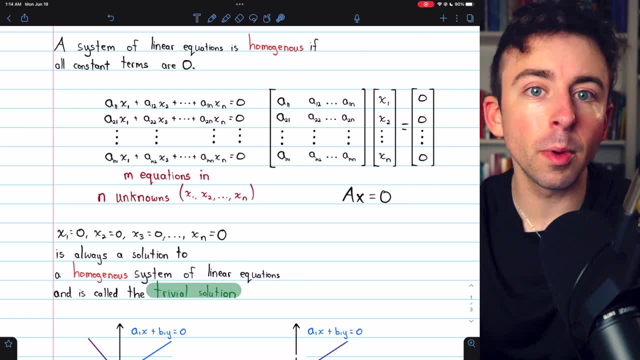 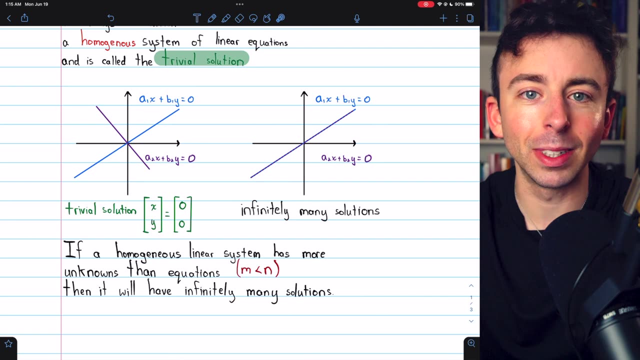 A homogeneous linear system of equations is a linear system of equations where the constant terms are all zero. Again, you know that a homogeneous linear system will have infinitely many solutions if it has more unknowns than equations, And we'll prove that next time. 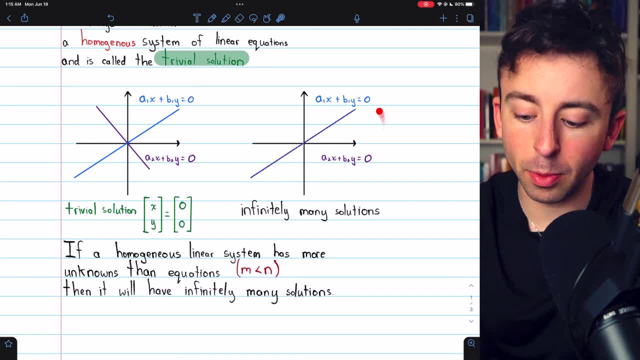 Link in the description. But keep in mind it's also possible, with the same number of equations and unknowns, to have infinitely many solutions. But a homogeneous linear system will either have infinitely many solutions or only the trivial solution of all zeros. 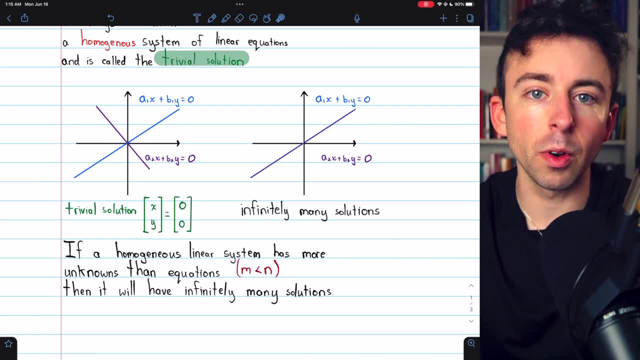 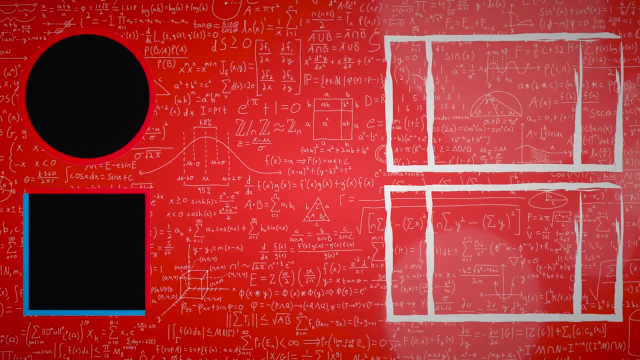 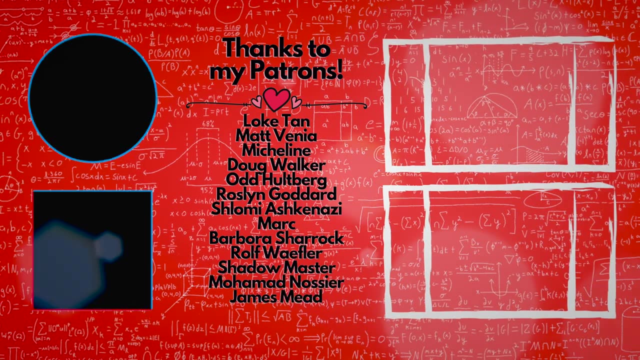 Let me know in the comments if you had any questions And if you find these linear algebra videos helpful. please consider supporting Wrath of Math on Patreon Link in the description. It's a huge help. Thanks for watching. Subtitles by the Amaraorg community.